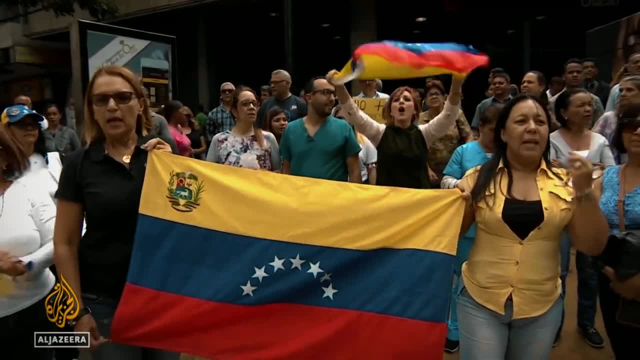 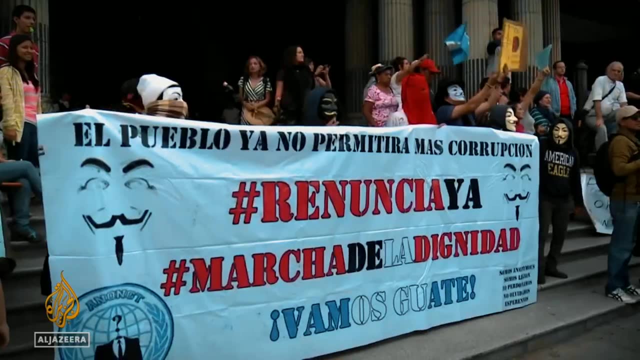 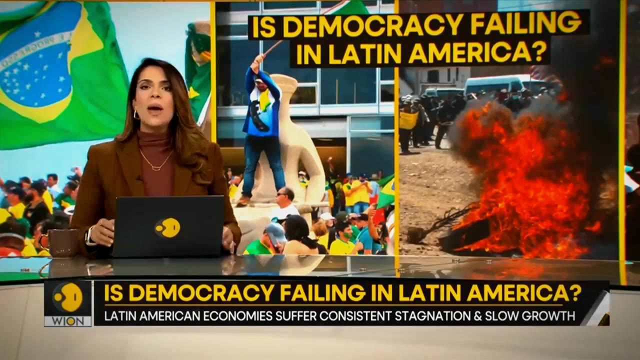 Additionally, political unrest can impede the implementation of crucial reforms and development initiatives as governments work to preserve stability and address citizens' immediate needs. This may result in a shortage of funding for essential services like healthcare, education and infrastructure, which could worsen the already existing economic and social. 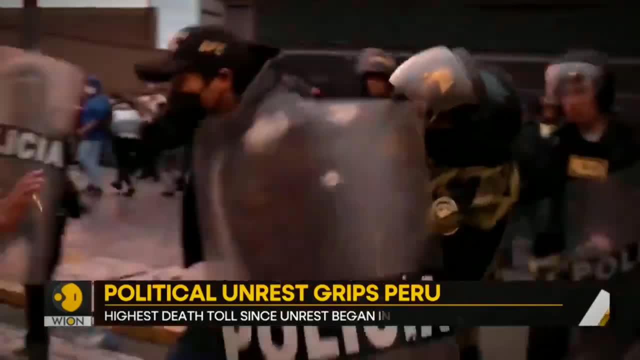 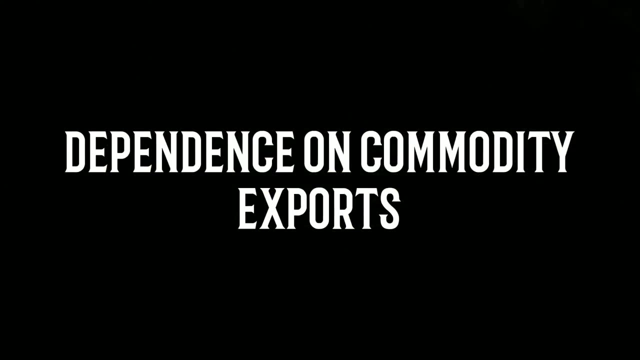 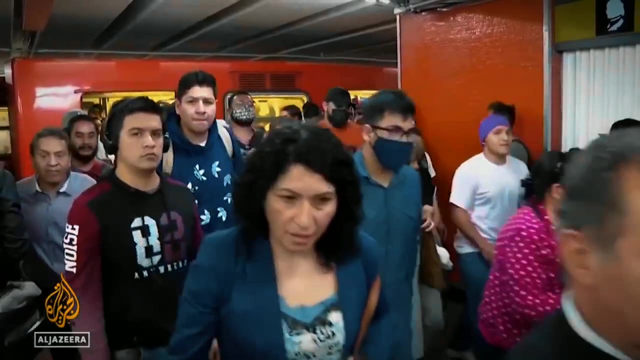 inequalities, Political instability occasionally even sparks armed conflict, which can have disastrous effects on the economy and society. 2. Dependence on Commodity Exports. Oil, minerals and agricultural products are among the resources that many nations in the region significantly rely on export. The depreciation of currencies and economic 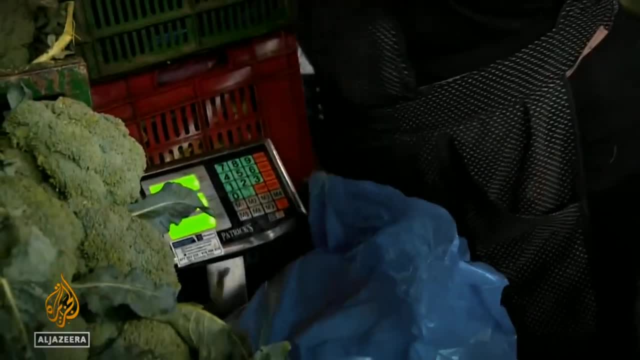 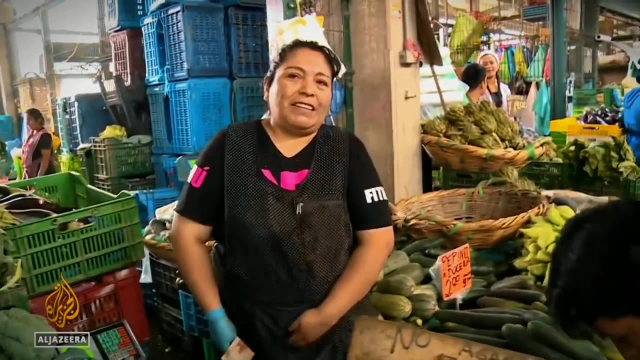 downturns can result from falling economic and social inequality prices for certain commodities. A small elite often gains from the export of commodities in many Latin American countries, while the rest of the population receives little benefit from this arrangement As a result of residents becoming dissatisfied with their lack of 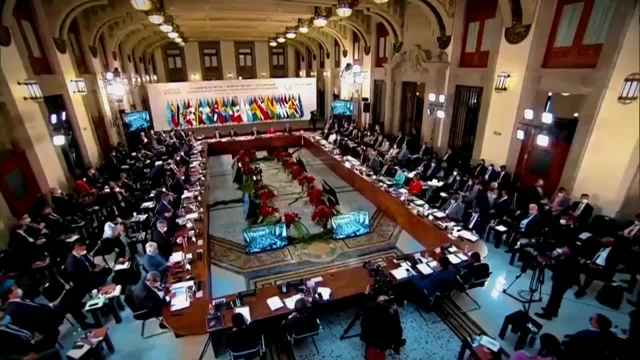 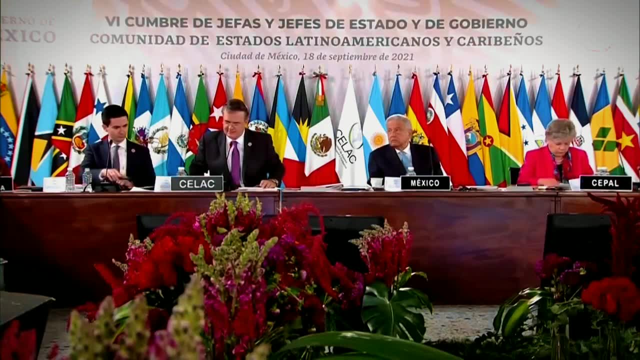 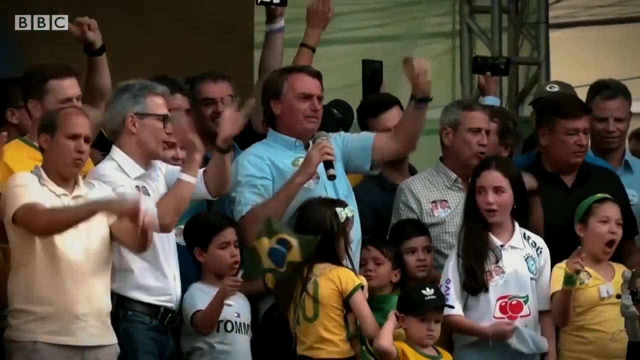 economic opportunity and political representation. there may be social unrest and political instability. Dependence on exports of raw materials can also result in a lack of economic diversification, which makes nations more susceptible to shocks from the outpouring of raw materials. 3. Economic Development Countries that depend solely on one product. 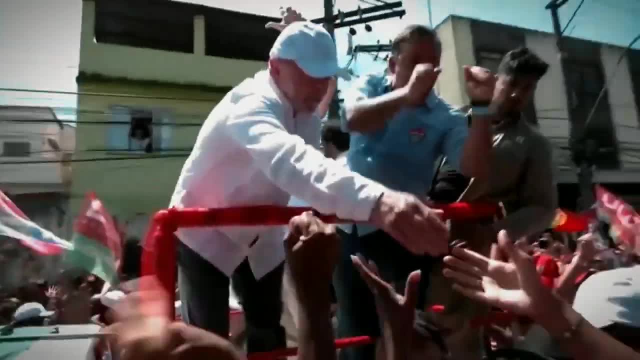 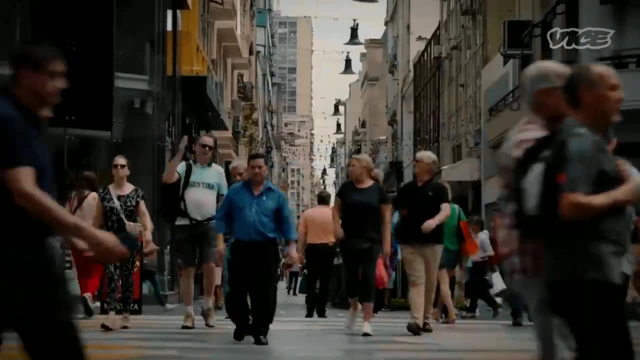 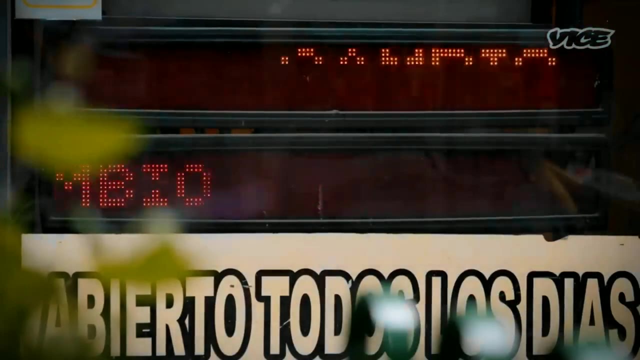 for their economic survival are vulnerable to the whims of the world market, which can be unexpected and turbulent. Making long-term investments and future plans may be challenging. as a result, Promoting economic diversification, making investments in infrastructure and education, and creating powerful institutions that can manage market risks are all necessary to address. 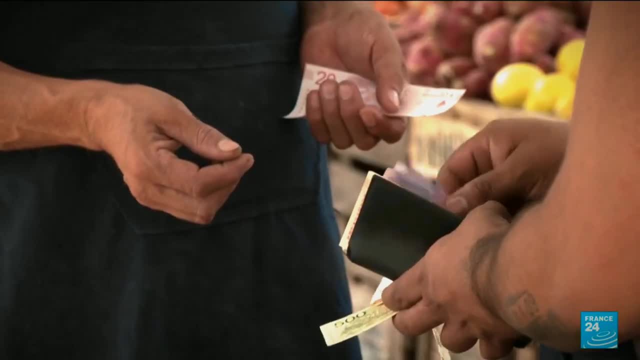 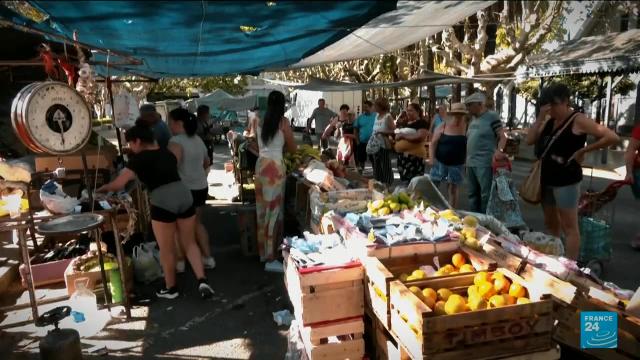 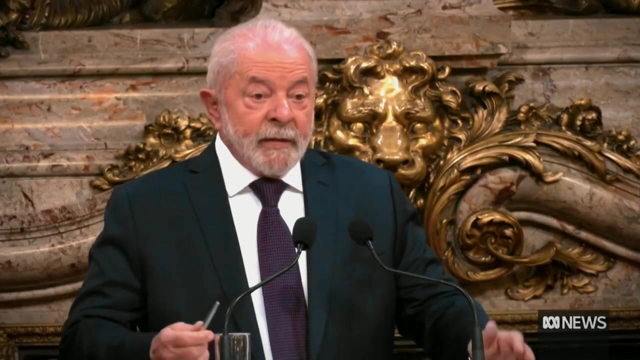 dependency on commodity exports. A dedication to inclusive economic development, economic growth that benefits all residents, not just a select few, is also necessary. 3. Debt Burden To finance public projects and social programs. many nations in the area have racked up considerable debt. However, a country's capacity to fund 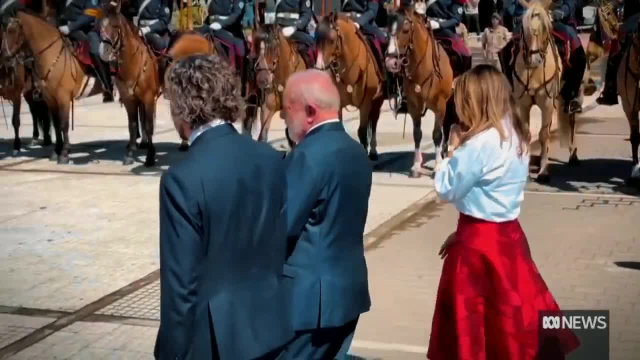 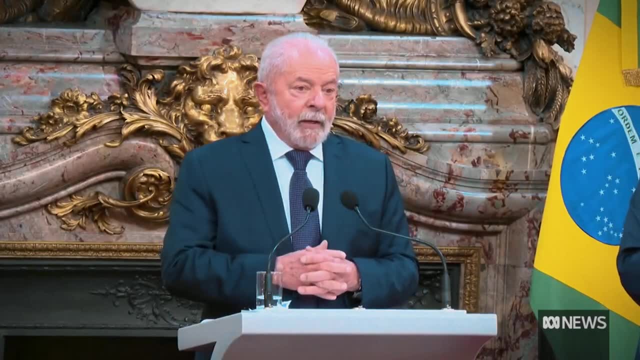 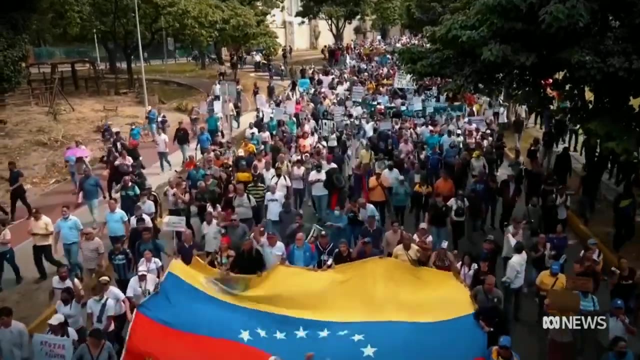 infrastructure and other economic development initiatives may be constrained by high levels of debt. There is less money available for crucial expenditures in infrastructure, health care and education. A country's capacity to fund infrastructure and other economic development is not limited by money, but by investment. 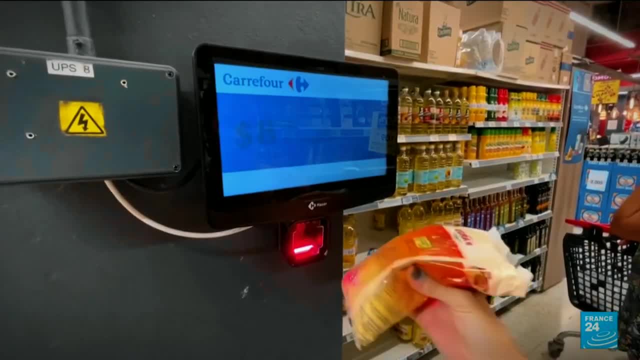 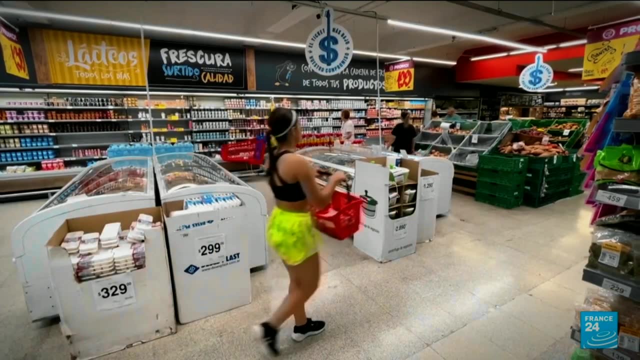 Gallup Ll tu goi. 40 interest rates, hundred dollar average. I look out in a isle in a country. all night Tower is so lonely for me and everything will get just a little too scared. I'm going to see what I can do in this nouble place. Then I will go find something to eat for lunch. No repız요. 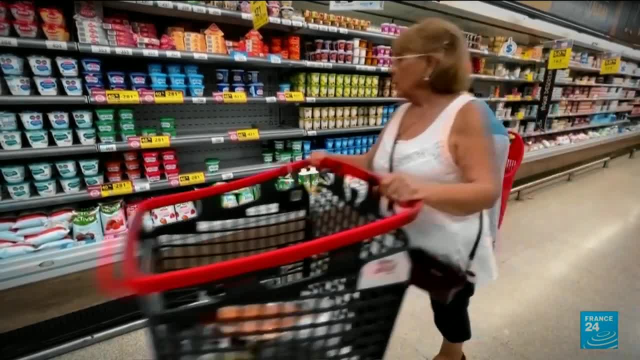 I went to bed for pizza before breakfast today. Bartend Radio is what I wasn't eating all night. the issue of excessive levels of public debt, Making difficult decisions about where to cut spending and prioritizing investments in vital infrastructure and social programs that have the 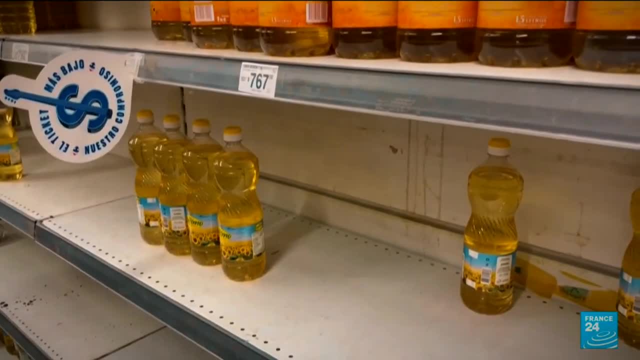 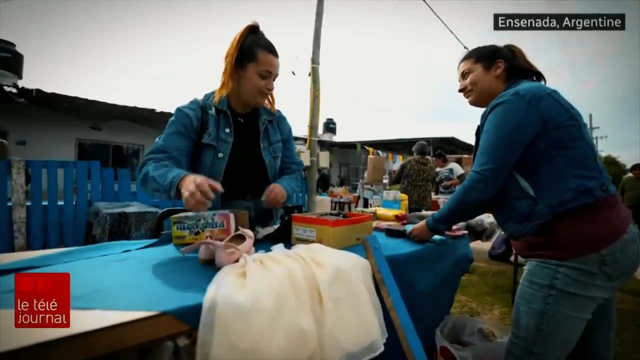 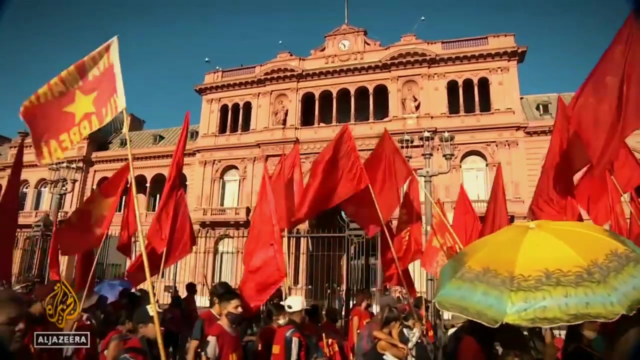 best chance of fostering economic growth and social development may be necessary to achieve this. Additionally, it might be necessary to look into alternative sources of funding that can assist nations in funding significant development projects without taking on excessive amounts of debt, such as private investment or international aid. 4. Weak Infrastructure. 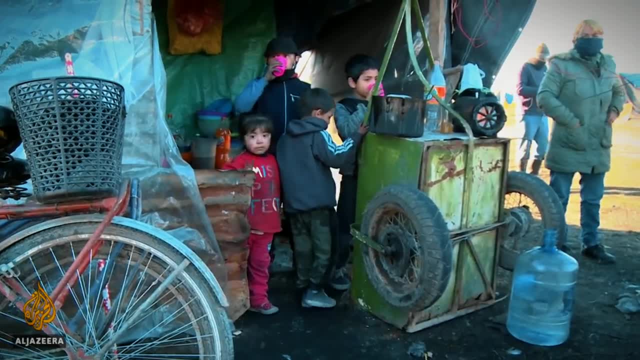 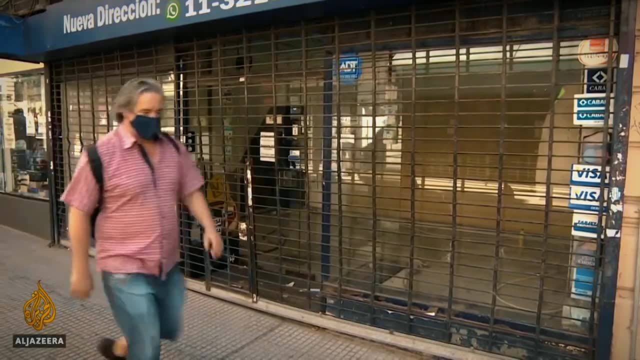 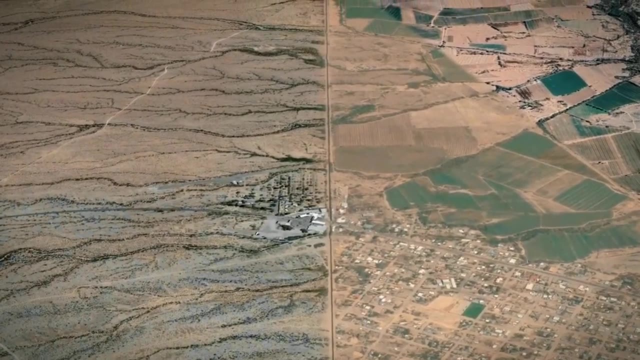 Many Latin American nations face significant infrastructure challenges that can hinder their ability to experience sustained economic growth and development. Businesses struggle to run effectively, get goods to markets and get the resources they need to expand if their infrastructure is inadequate. Additionally, inadequate infrastructure can restrict access. 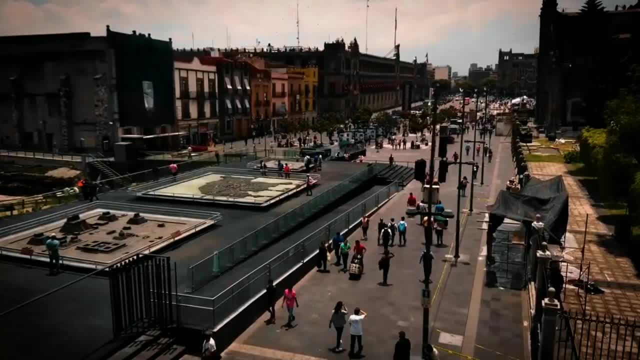 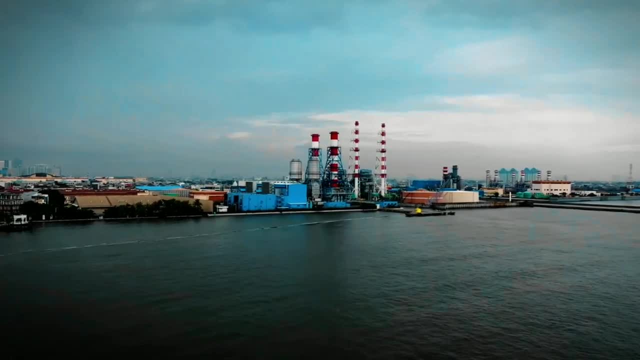 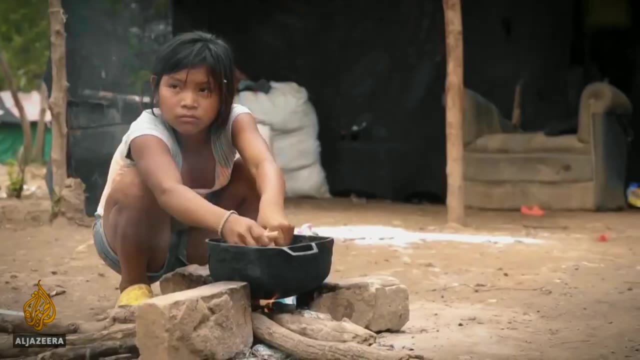 to essential services like safe drinking water, Sanitary facilities and healthcare, which can have a negative effect on the general well-being of the population. Additionally, a lack of infrastructure makes a nation more susceptible to environmental shocks, like natural disasters, which can have catastrophic effects. 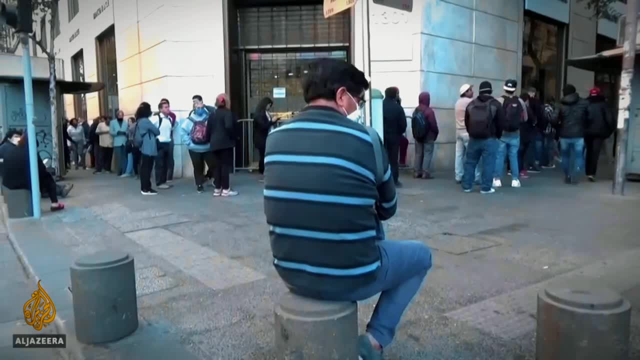 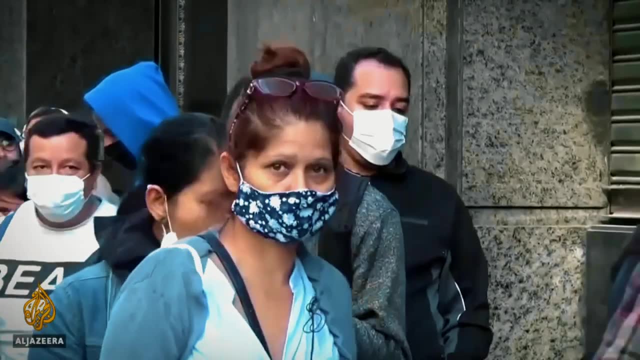 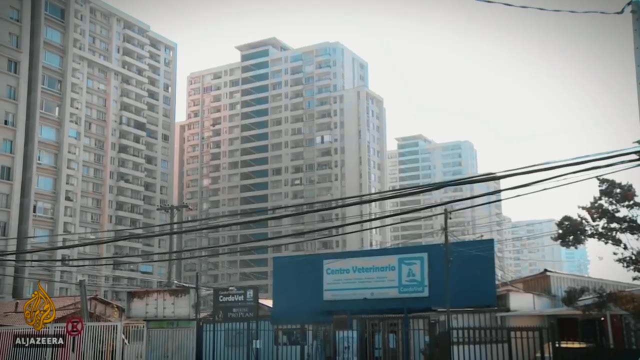 on the economy and society. Significant expenditures must be made on water and sanitation systems, energy sources, transportation infrastructure and other vital infrastructure in order to address deficient infrastructure. 5. To Acquire a Good Infrastructure: To acquire funding and technological know-how. this may necessitate collaborating with partners. 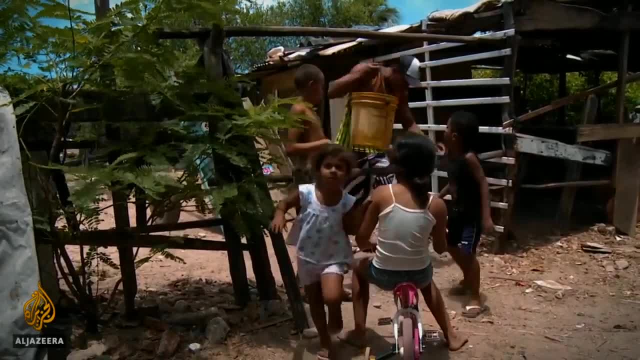 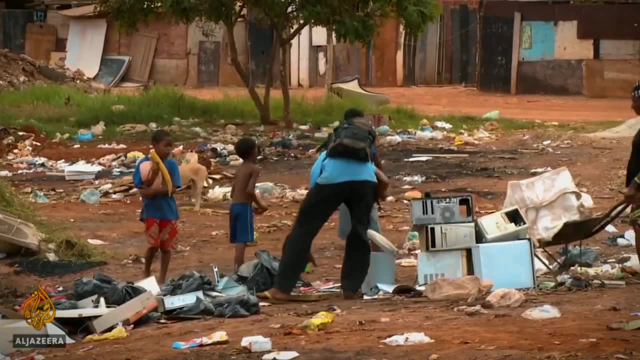 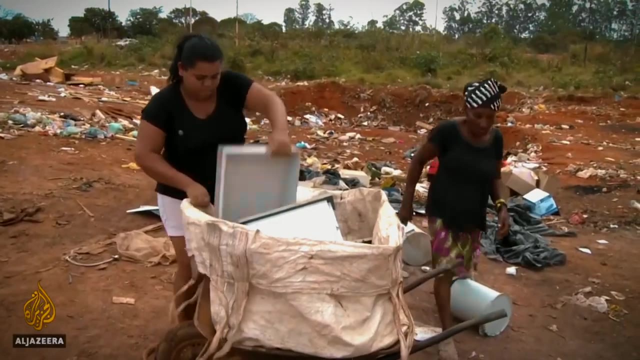 in the corporate sector and international development organizations, Making it simpler for private sector entities to invest in infrastructure projects may also need major regulatory reform For the purpose of fostering economic development and ensuring that all individuals have access to the fundamental services they require to live healthy and productive lives. it is 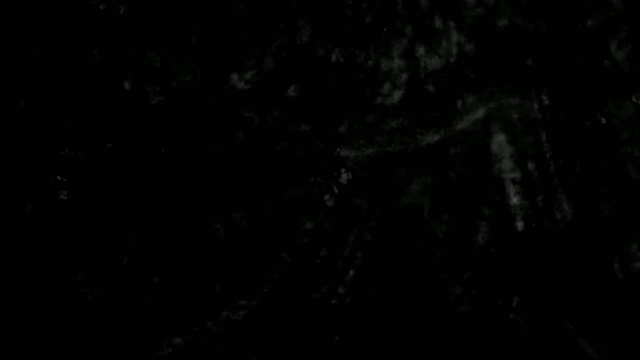 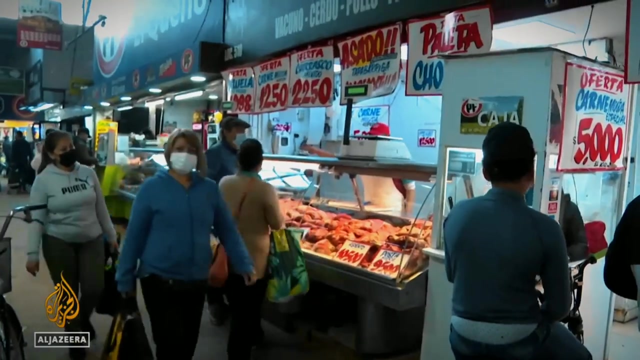 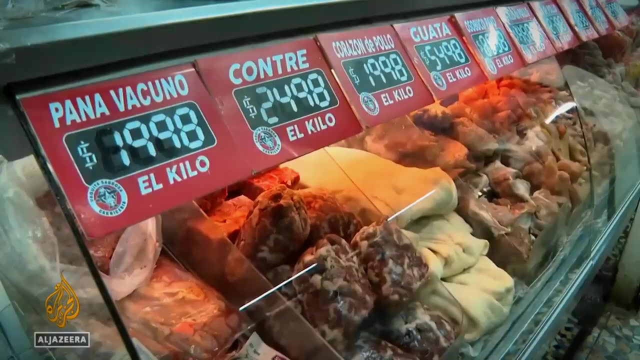 crucial to invest in a robust infrastructure. 5. Income Inequality. Latin America faces a wide-ranging problem with income inequality, which can be detrimental to both social progress and economic development. Economic options for the rest of the population may be restricted when income is concentrated in the hands of a small elite and social 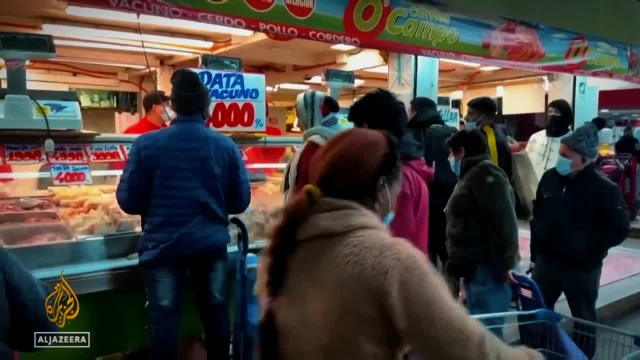 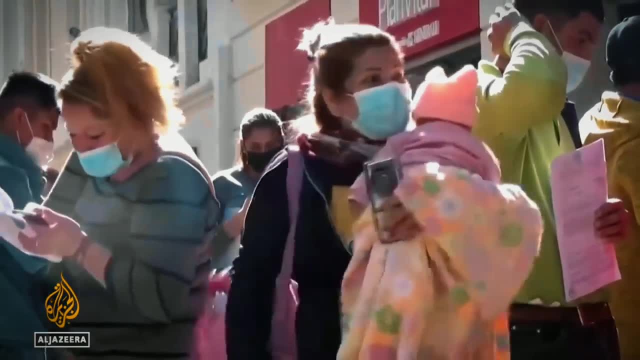 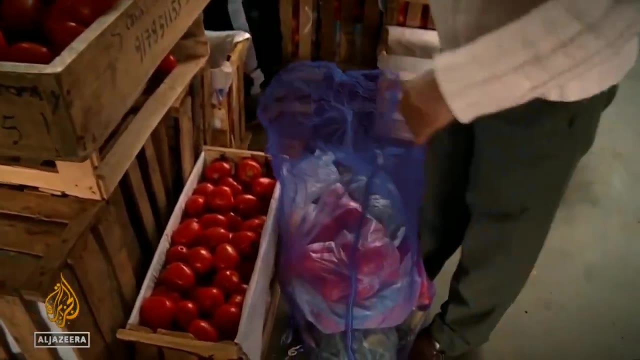 and political tensions may develop that may spark instability and violence. Additionally, access to essential services like healthcare, education and other necessities may be restricted as a result of income inequality, further entrenching poverty and reducing opportunities for upward mobility, Because many people cannot afford the goods and services that businesses produce. high levels of income inequality can also reduce consumer demand. A multifaceted strategy that incorporates both redistributive laws and investments in human capital is needed to address economic disparity. This may entail progressive tax laws that make sure the wealthiest pay their fair part, as well as social safety necessities. 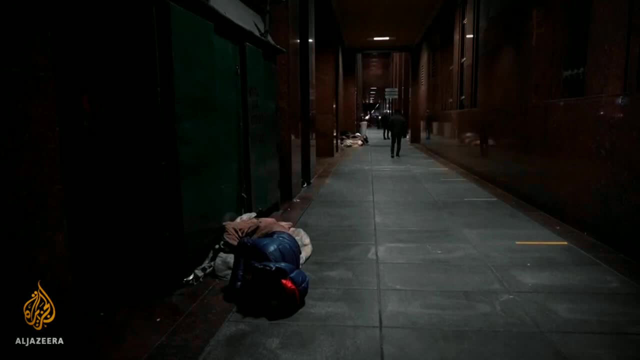 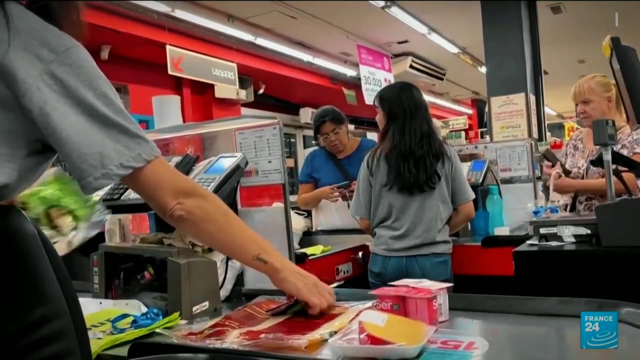 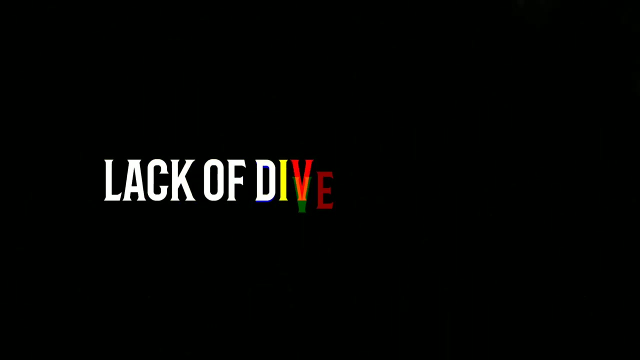 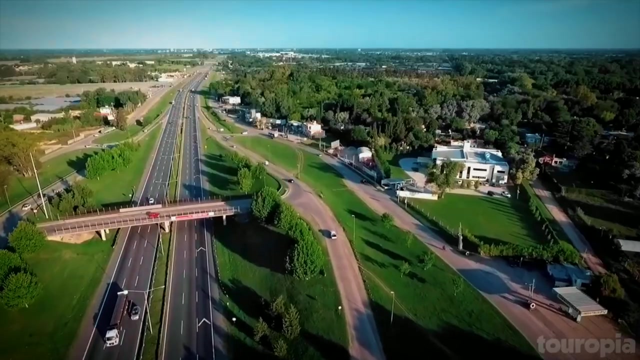 6. Increasing Income Inequality. Let's look at the five key factors that apply to our economic and social wealth. • Lack of diversification: Many nations in the area rely heavily on a small number of key industries like mining, agriculture or tourism, making them susceptible. 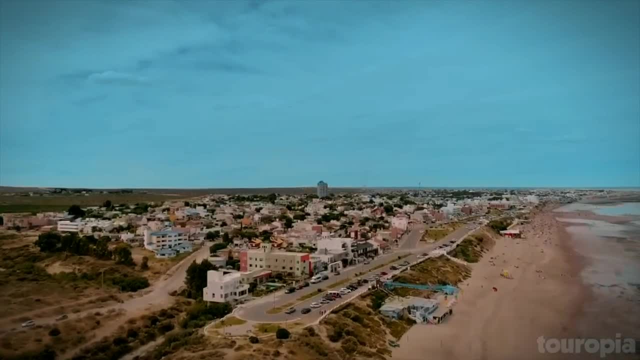 to outside shocks and market floods. Serbia, which is majorly dependent on two major mining HORNA, is being a centre of our economic and social output. During COVID-19 pandemic, the country was able to stay in fluctuations. Countries that depend on a certain commodity for a sizable share of their GDP. for instance, may experience economic downturns and currency devaluations when the global market for that product drops. Additionally, a lack of diversification can restrict opportunities for entrepreneurship and innovation and lead to a business environment that is disproportionately dependent on a small number of major players, Promoting a more dynamic and competitive business. 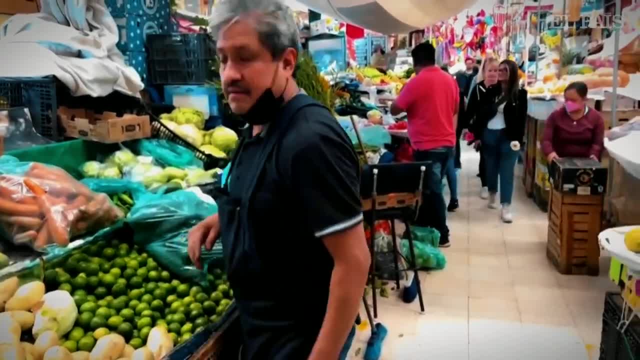 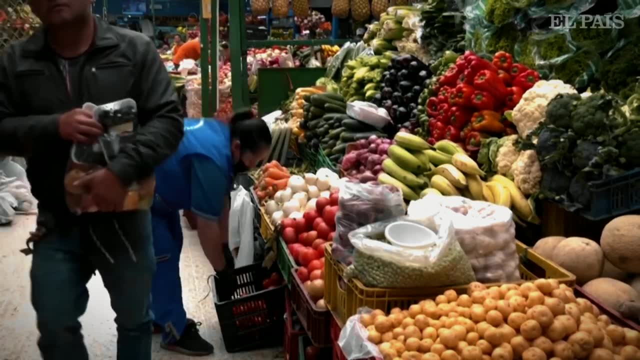 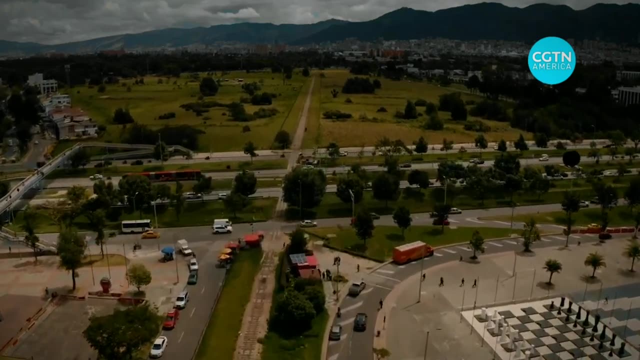 climate and making investments in education and human resources are necessary to address the lack of economic diversification. To achieve this, it may be necessary to assist small and medium-sized businesses, encourage innovation and entrepreneurship, and invest in education and skill development to develop a workforce that is more varied and talented, In order to stimulate 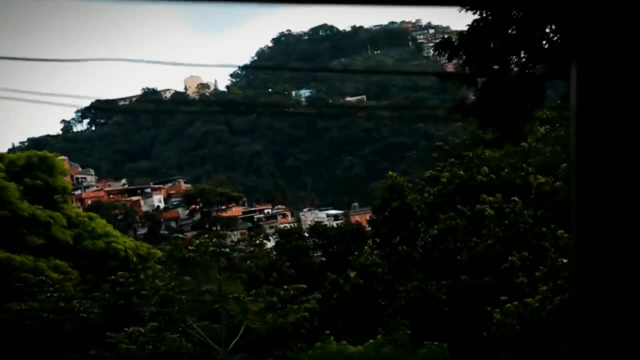 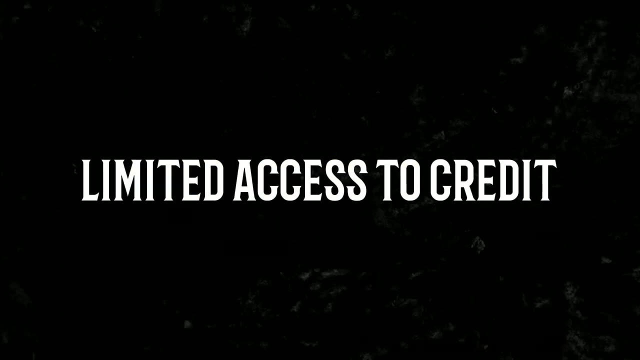 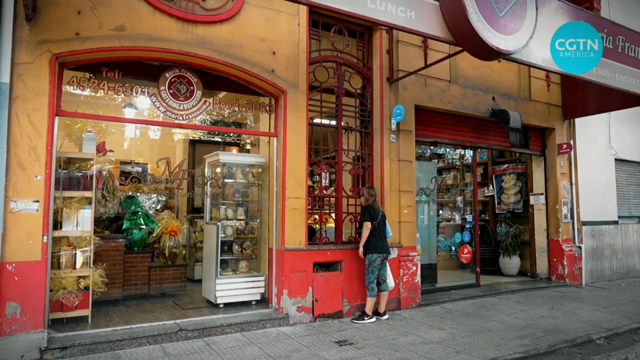 investment in a wider range of industries and to make it easier for firms to start and flourish. regulatory change may also be necessary. 7. Limited Access to Credit. For many Latin American nations, having limited access to financing is a major problem, especially for low-income groups and small and medium-sized firms, SMEs. It is challenging for